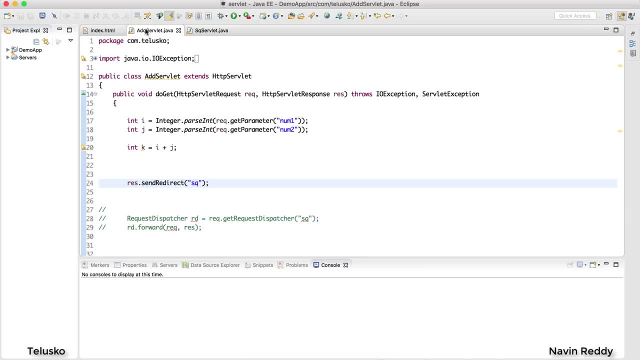 third servlet. it will be there for you. So what if you can put your data into session? So once you put your k into session here, you can use that session value in the next servlet. How do we do that? As I mentioned, session will be given by tomcat. we just have to get. 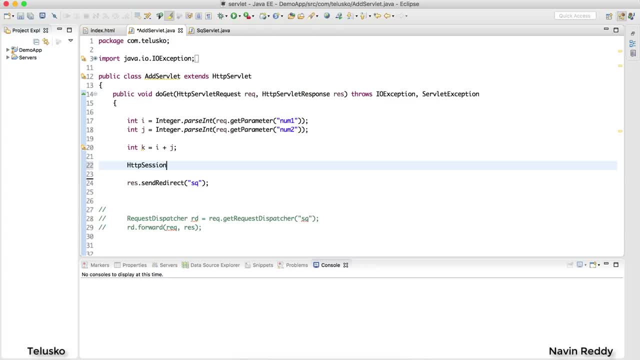 the hold on it, And the way you do that is by using http session. So http session is an interface. We just have to say http session session and, as I mentioned, the object will be given by tomcat itself. You simply have to say requestget session. we just have to. 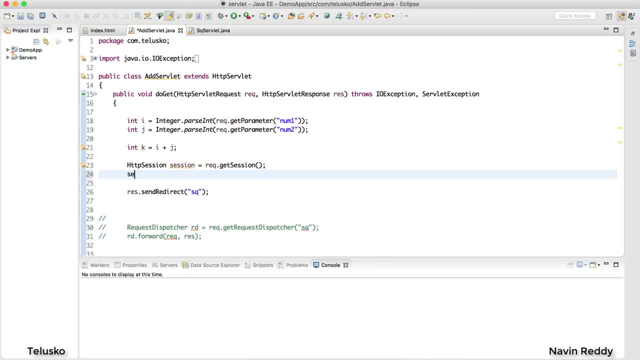 get the hold on it And once we got a session object with us, we will simply say sessionsetattribute, because session will be there throughout your visit to the website, right? If you go to add servlet, if you go to sql servlet, even after some time, if you go to some other page which is the 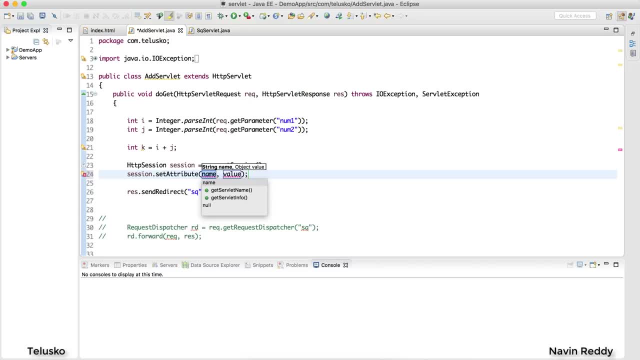 same application. the session will be available for you, provided you don't close the session, provided you don't remove the value from the session. We can do that, by the way. So we will say sessionsetattribute and I would say the value is going in a format of k and 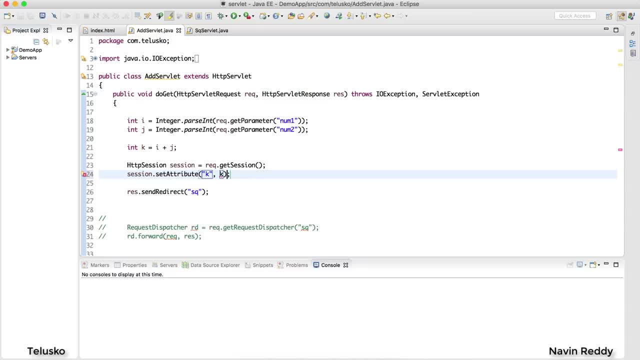 the value itself is k. The value which is k is stand for attr couple, which is k and the value is k. How do we access that here? how do we fetch the value Now? of course we are not sending data into request object. We are sending data into a session. So the way you fetch the value now is by saying: 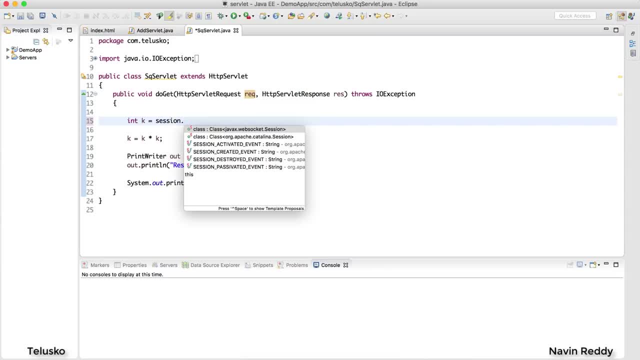 the way you fetch the value now is by saying: So, remove that, We will say sessiono. We have not. instead, we have not given the offence session, we have not declared it here. So let's say HTTP session Session. equal to the same thing. Requestget sessionattribute by something. 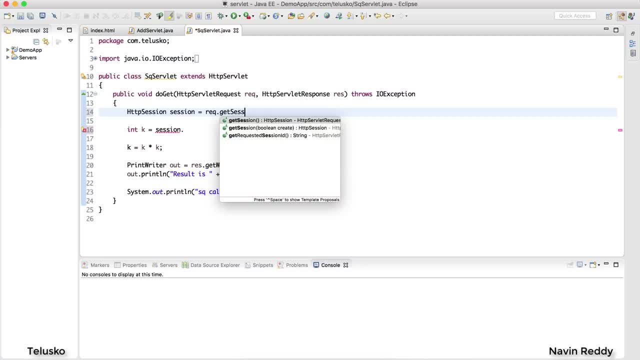 which is klasssetattribute. I will remove that now and we will download and install session. глав disorders poly chem. It is not in the format of songs or songs, just decade period. Você pode usar is 50%. is that session and once we got a hold on it, once we got the hold on the session, object, i would say session. 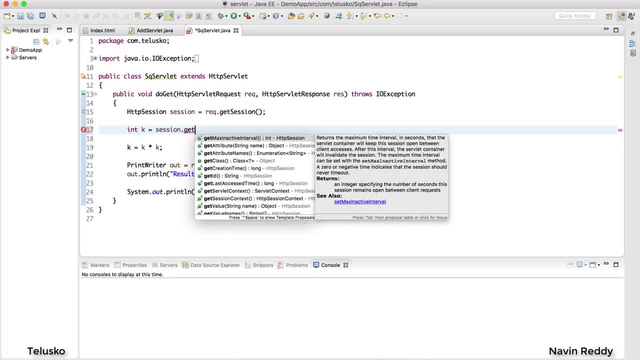 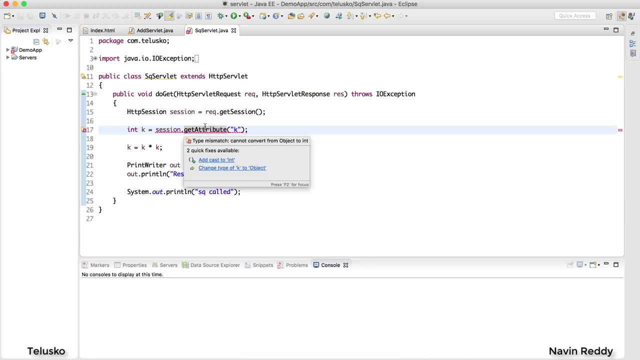 dot. get inside. add sublet. we have said set attribute. here we have to say get attribute. it's that simple. and here i would mention: i want k. okay, now there's one issue. when you say attribute, it means it will return you the object. we don't want object. what we want is the int format, right. 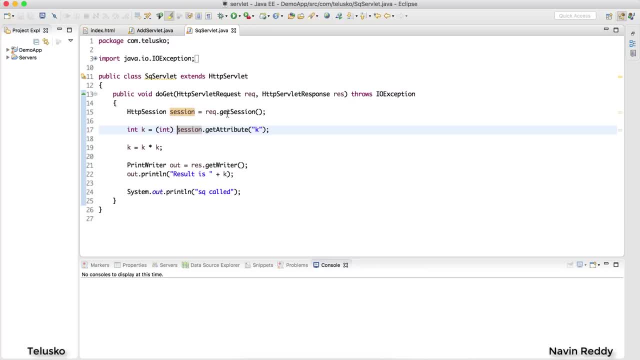 so we'll simply type cast. it will say int and we are done. so this will give you object and we have to convert that into int. we just simply type casting it again we can. we can say integer percent as well. we just have to convert it into string. but multiple steps, right? this is simple, we see. 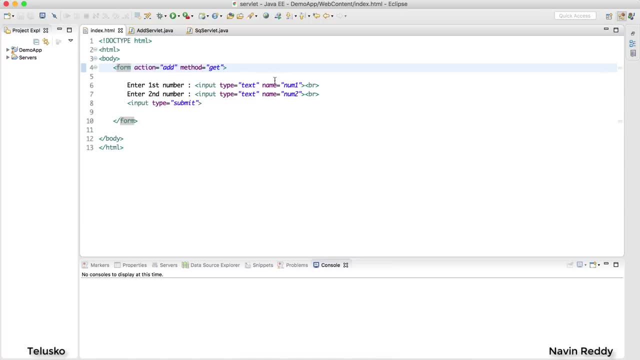 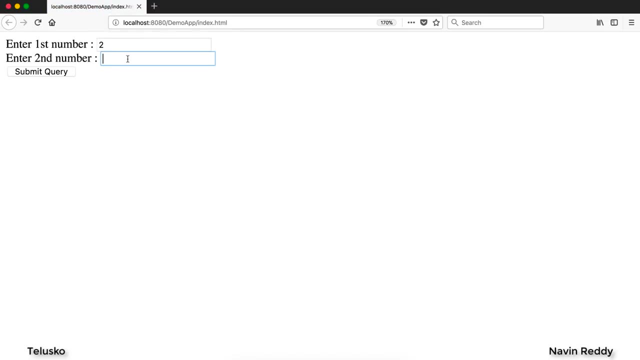 we can simply type cast it with int. now this should work. let's verify. i will go back to my html. i will say: write like run as the non-server. so it is opening my firefox and here i would say two and three, which is five, into two, which is 25. answer should be 25 and we got it. can you see that? 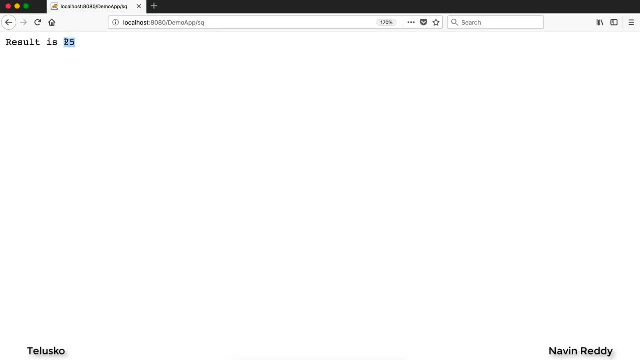 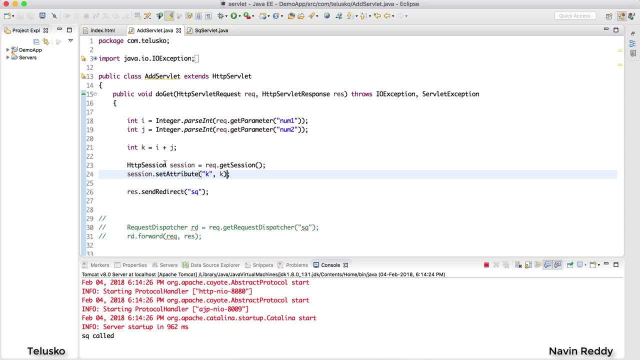 we got the answer. so first it is adding those two values and then it is. it is finding a square of a number. quite simple, right? so we can use session as well. now, as i mentioned, the data will be available in this session for you throughout, provided you don't delete this data from the session. can we really do? 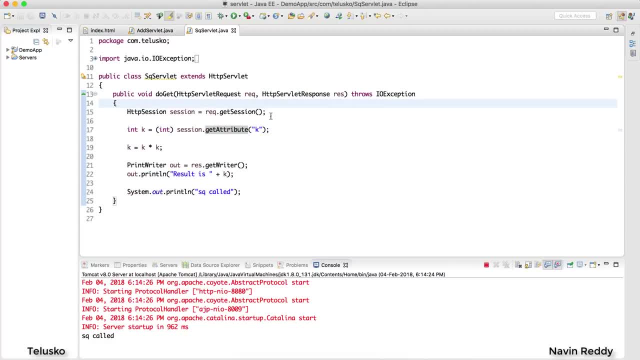 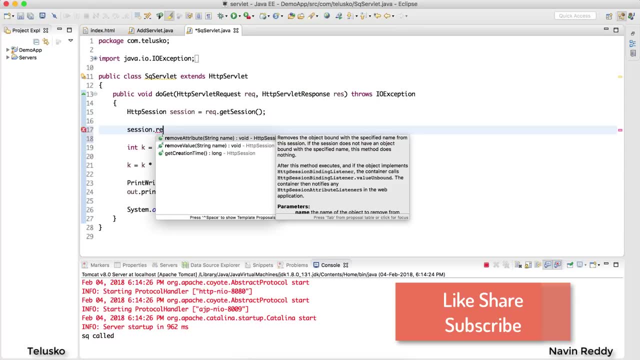 that? yes, we can. actually we can delete data from a session, so we can. once you've got the hold on it, we can say: session dot, there are. there's a way you can say: is it remove attribute? yes, you can say that we have remove attribute and you can remove k here now, once you remove k, of course. 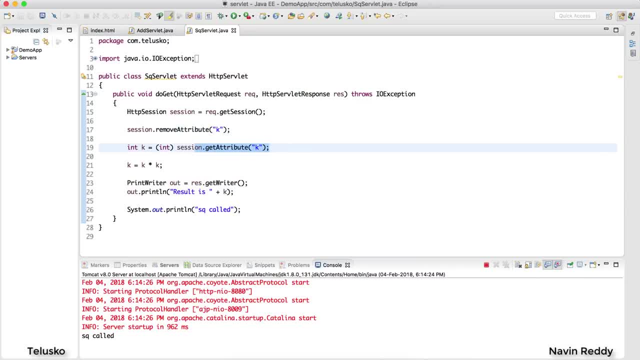 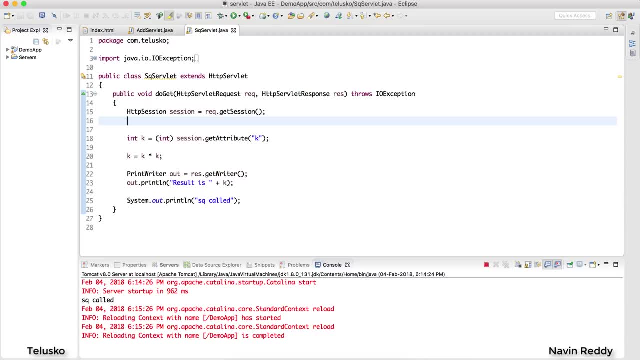 you cannot fetch the value. so you can fetch this value only when you have the value of the session. so using this, you can removed. that's how you can use session now. normally you can use this usion cru maintain login. so lets say you log in on your website and you want to verify if a user goes to another page and if you want to verify the users are already logged in, you can. you can maintain the data in the session. that's what we do, but this looks cool. right, session looks cool. do we have some other way? like we'll be working on session more in the future topics once we come to jsp. but can we do something more here? and the answer is yes, u can ruined session. one option now by the U Kolbin sait which we'll be using. 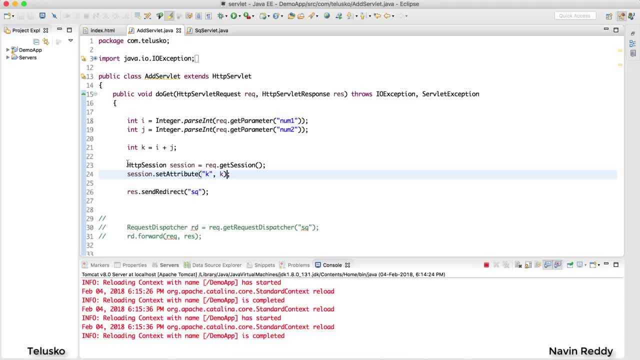 yes, what we can also do is we can use cookies as well. so the way we have session, we can also use cookies. now how that works. so what i will do is i will not use session anymore, let me remove session. let me remove session from it everywhere. i want to use cookies here. so i would say int k again. 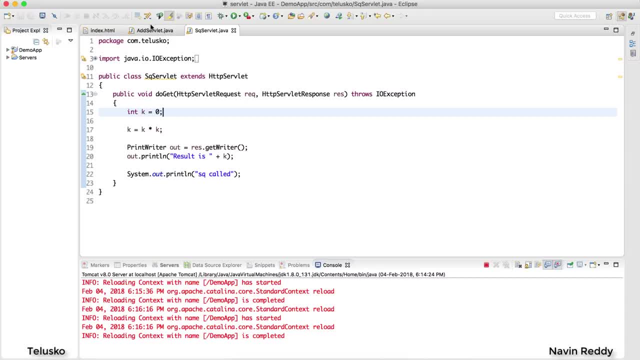 initially i would say zero. how do we do the same thing with the help of cookies? let's get back to add, and here i would say i want to work with cookie. now, what is cookie basically? so, whenever you send a request to the server and a server will send you a response, now in that response, 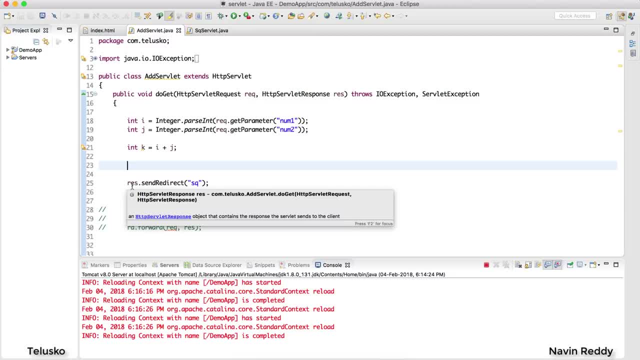 object. so the response object, which is coming from the server, will have a cookie and then when you, when you send a request to sql server, you can send the same cookie again. so difference would be: the cookie is coming on the client side and then you're again sending the cookie to the server. 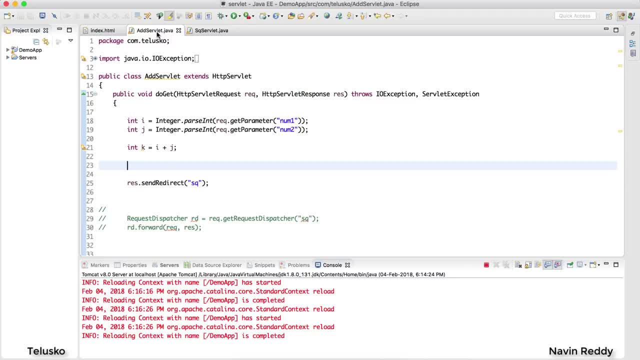 now, if you want to imagine this, imagine you're going to a shop to buy something, or, let's say, if you are going to a restaurant, or if you're going to a restaurant which provides your self-service, where you have to buy the product first, you have to pay the amount and 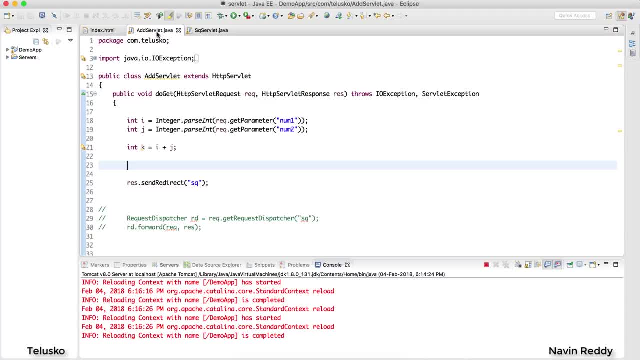 then you will get the, get the dish or whatever you want to eat. so let's say you, you want to buy something which which cost you around, let's say, 50 bucks and you are giving 100 bucks, so you don't have a change with you. so the, the product cost you around 50 bucks, but you're you're paying 100 bucks. 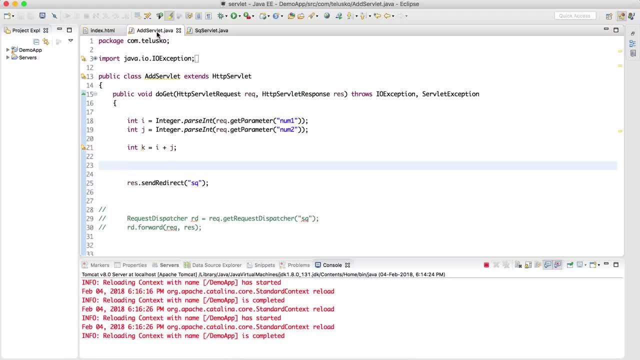 and the shopkeeper says, or the restaurant person says, hey, he don't have a change. now, of course you don't. even you don't have a change, he don't have a change. what you will do, he will say: okay, wait for some time. once i got the change, i will give it to you. you go back to your. 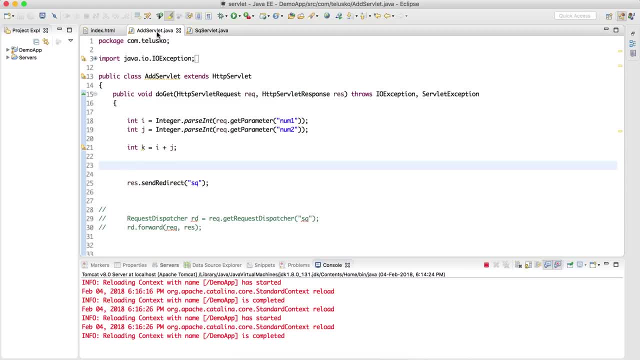 seat and then, after half an hour, you go back to the cashier and say, hey, i want 50 to 50 bucks back now. will you remember you? of course not right after half an hour. he may forgot who you are. so in the earlier scenario, what you should have done is the moment he says: hey, wait for 30 minutes. he. 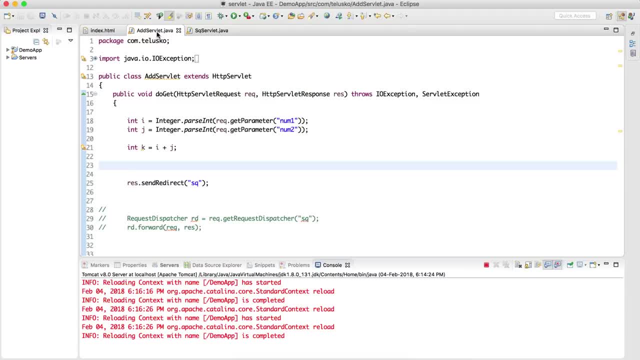 will give you a token. on that token it will, it will write: he will write 50, which means when you go back to him after some time, you can show that token which says 50 bucks, which means 50 bucks- that's a cookie. when you go for the first time, he will give you a token so that when you go back, 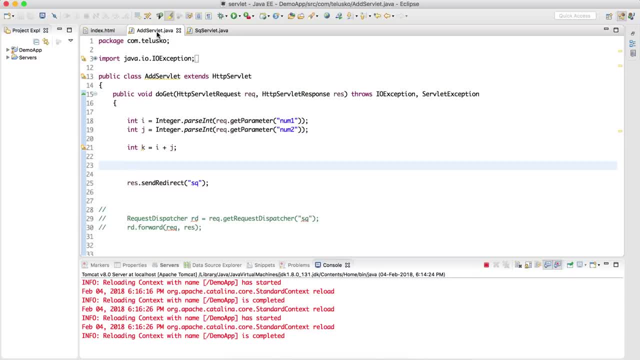 to him after some time. you can use a token. i hope you understood something about that example here. i will try to implement that with the java code. so i would say cookie, that this is how you create a cookie. you say cookie. cookie basically belongs to java x packet, java x dot serverhttp and i would 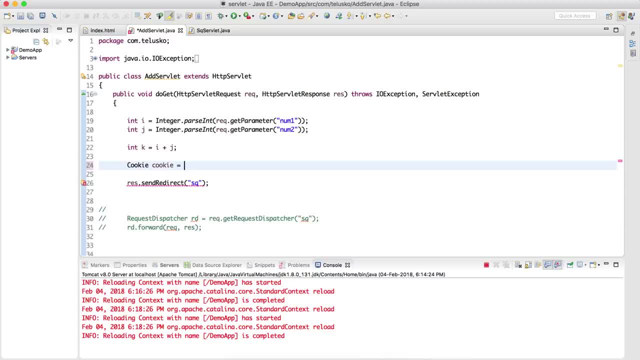 say cookie equal to how do we create a cookie. it's a class, basically. so we can simply say new cookie. first parameter is the name of it. i will say k and the value of it, which is k as well. so i'm have a name which is k and the value is k. we got a cookie as we got our cookie. we cannot simply pass k here. 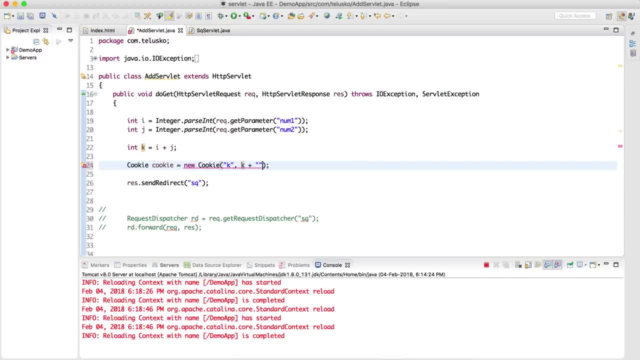 it should be string. how do we convert this k into string? we can simply append a double quotes, right, so integer. append double quotes is string. now, once we got this cookie, we just have to add this cookie to the response object so that it will go to the client. i would say: response dot, add cookie and. 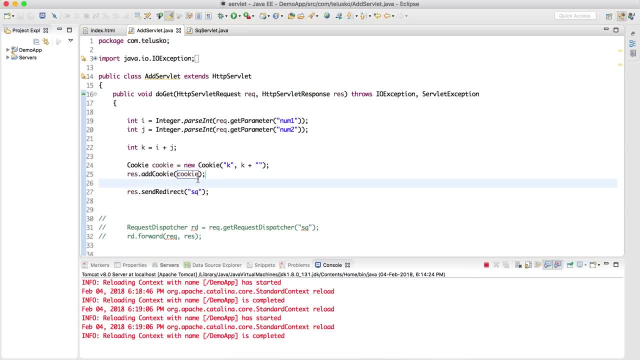 i'll pass cookie. that's done. we are sending the response to the client and we are sending the cookie to the client now. this means this add servlet will send the response to the client and client again will send a request to sq servlet. now when a client send a request to sq servlet. 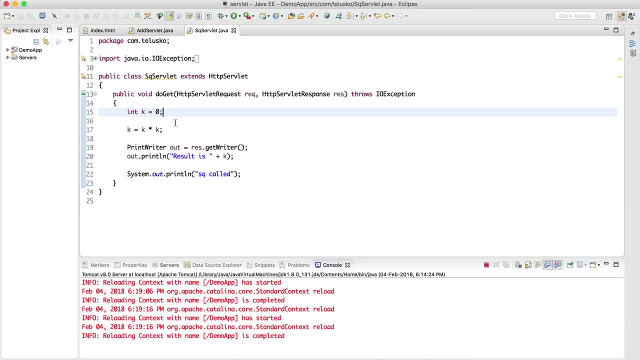 again, it will send the cookie as well. oh, that means we have to first accept the cookies, and the way you do that is by saying: oh, how do we do that? so when a servlet send a response to the client, it is response object: right, and next time when a client send a request to the sq servlet, 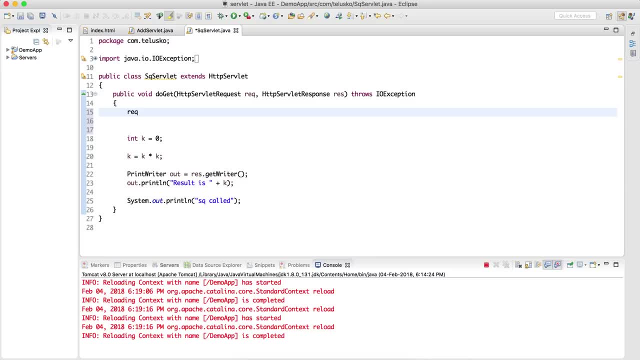 that means the the cookie will be coming in the request object, right? so i will say r e q dot. do we have a get cookie method? so i will try to get guess that. oh, we don't have get cookie, we have get cookies. that's weird. why get cookies? why not get cookie? it is possible that on the client side you 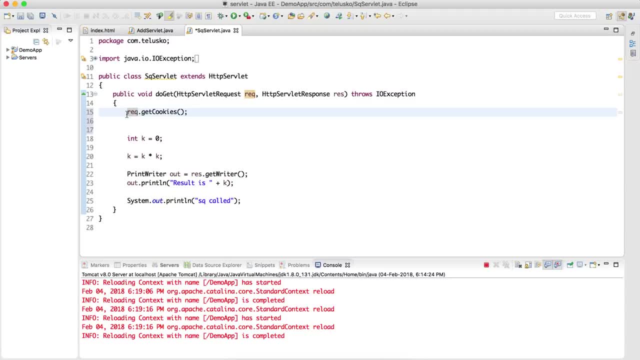 don't have one cookie. you have multiple cookies, quite possible. right, we don't want, okay, so it will give you all the cookies. because client even don't know which cookie you need. so client says, hey, i will give you all the cookies. you figure it out what, which cookie you want to give you. 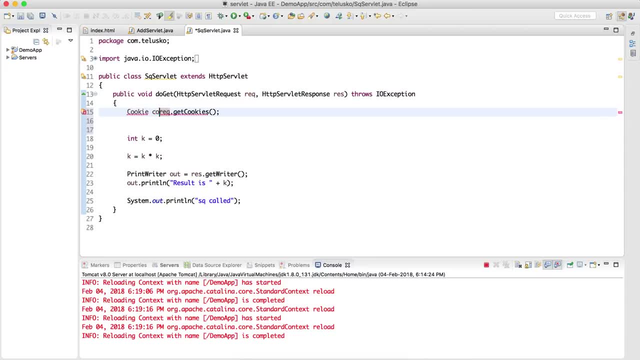 want. okay. so since client is sending all the cookies, i have to use an array of cookies. so i would say: cookies array equal to let me import the package. as i mentioned, we are not getting one cookie, we are getting cookies. so that's why we have an array, and from this array i want to fetch. 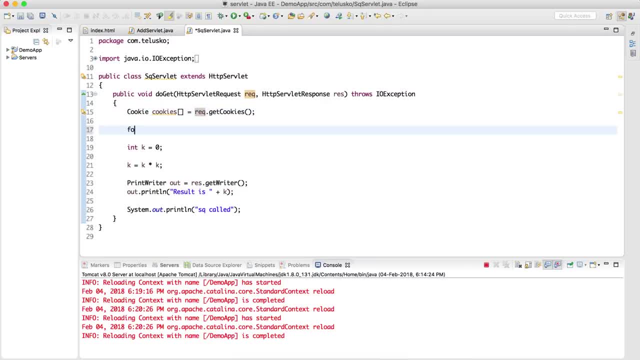 the cookie which i want. how do we know which we, which i want? for that i will use an announced for loop. i would say for: in fact, you know, i will just declare this variable up here so that i can use it later. i would say for enhance, announce for loop works something like this. i would say: 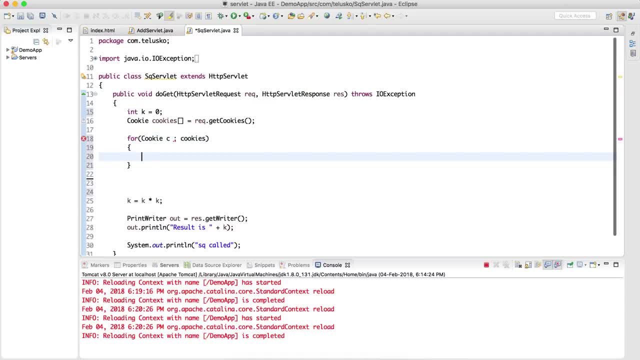 cookie c equal colon cookies. it will give you, it will run a loop through to all the cookies and then i would say what, how do we fetch a cookie now? so i would say, first of all i want to know which cookie i want. so i would say, if the cookie name- so i would say cookie c dot get name, is it the? 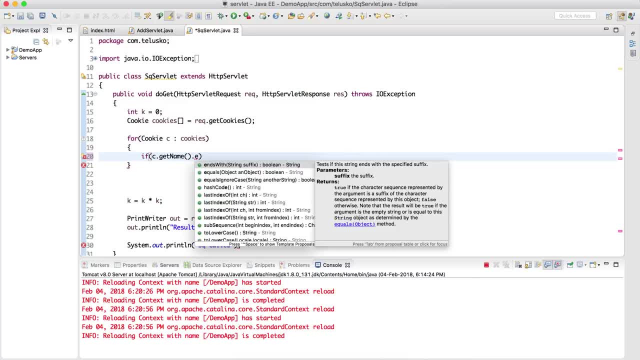 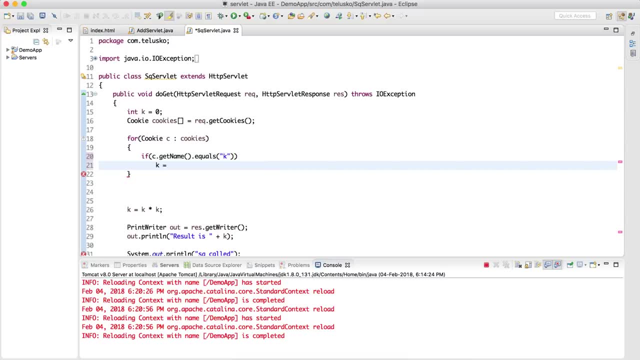 uh, yeah, so we have get name if the name equals k. that's what we want. to compare right. if name equals k, this is our cookie. i would say k equals to c dot, get value. so we don't want all the values, we want only value of that cookie which has a value, which is the name of. 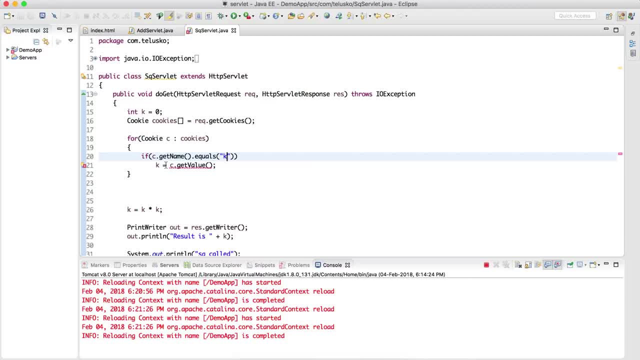 with the name with k. okay. now it says: get value will give you object. i don't get value. give you what string we have to convert that into integer. so i would say: integer dot percent. okay, so this is how we can fetch cookies and let's verify if it is working. i'm not sure. let's run this code. 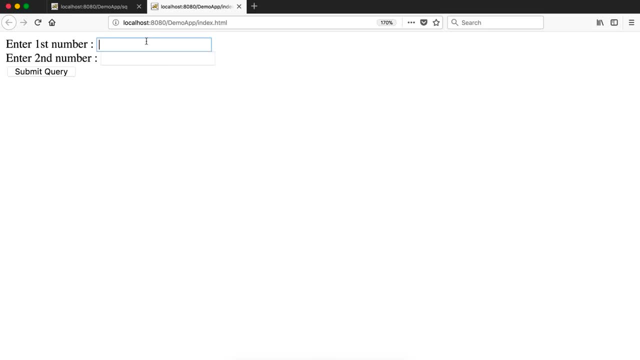 let's verify. i would say restart. so here it is asking for two values. i would say eight and six, and if i say submit, you can see we got 196, which is the square of one of square of 14. so it works. so, yes, you have multiple options. in the last video we have seen. 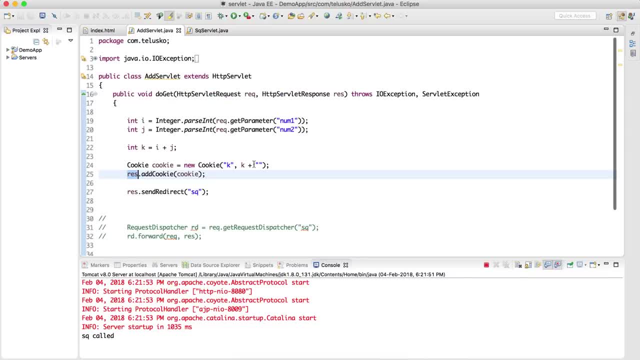 url rewriting. in this video we have seen how do we use session. i know how do we use cookies to send this data. uh, let me know. if you have not understood the example here of cookie, i will try to create a theory video where i will explain how that cookie flows from a client to the server. 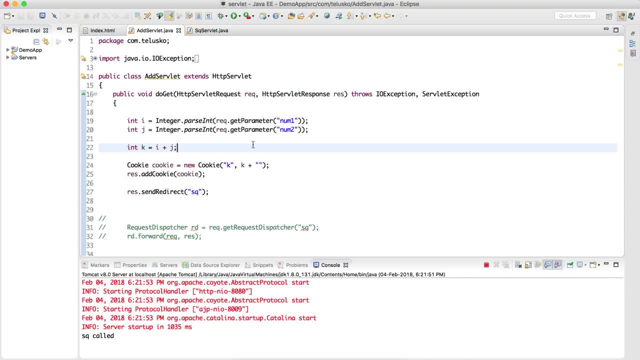 so that's it from this video. we have talked about session. we have talked about cookies. i would also recommend you to practice this code. try some, try different examples, not just addition of two numbers. you can also try login, username, password- uh, you can also try to use, or maybe you can. you can do some other operations as well. so try it out, let me know. 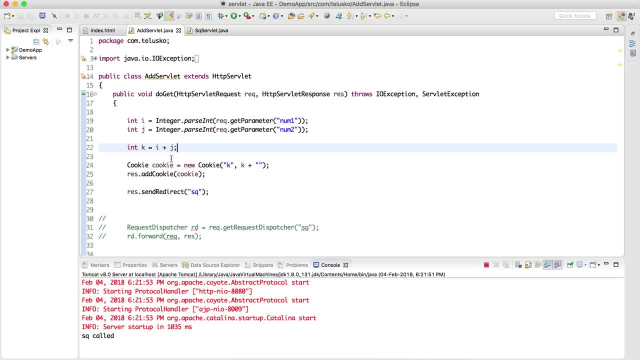 in the comment section if you enjoyed this video. waiting for your comments, and do like the video if you enjoyed it. thank you so much for watching everyone.